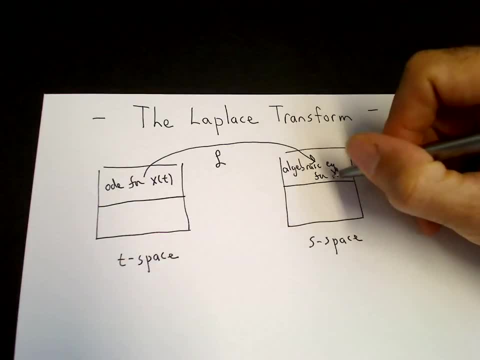 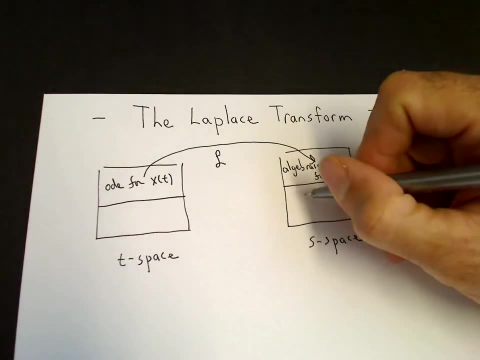 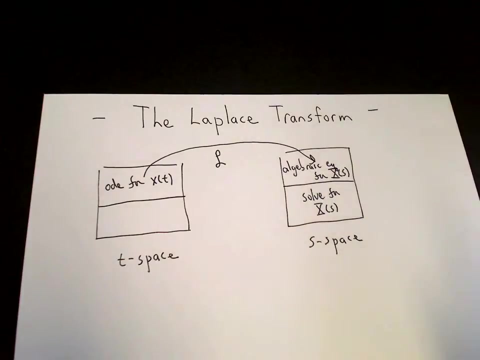 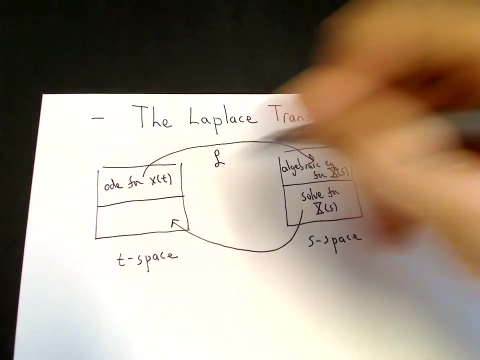 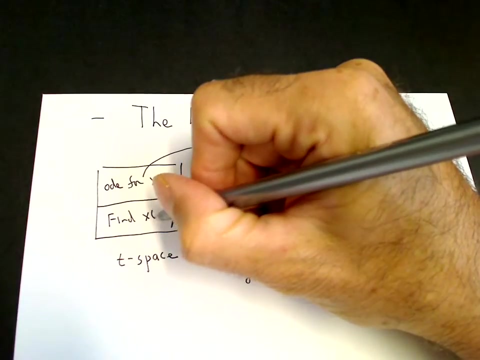 Equation for x of s right. And then in s-space we solve for x of s, which is easy because it's an algebraic equation, And then we transform back to t-space with the inverse Laplace transform to find x of t. 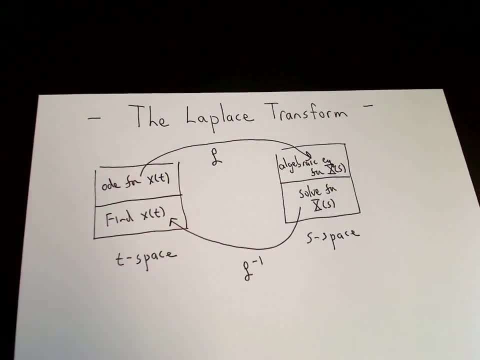 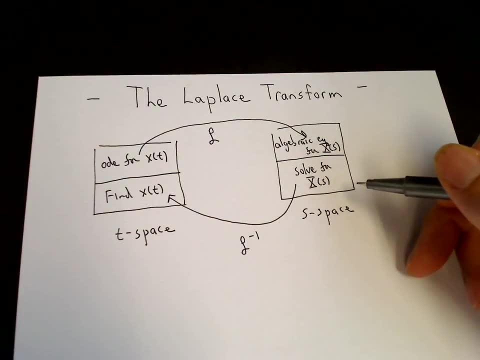 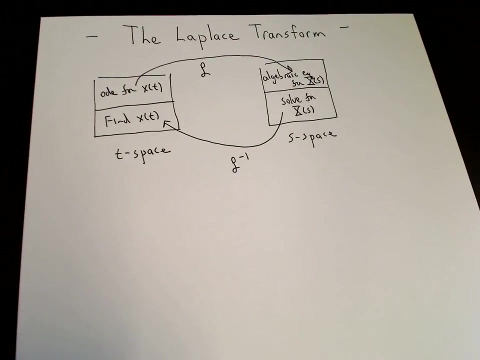 Okay. So the technique is such that if the equation is easier to solve in s-space, then we transform the ODE to s-space and solve the equation and then transform back to t-space. So the question is then: what is the Laplace transform that enables us to do this? 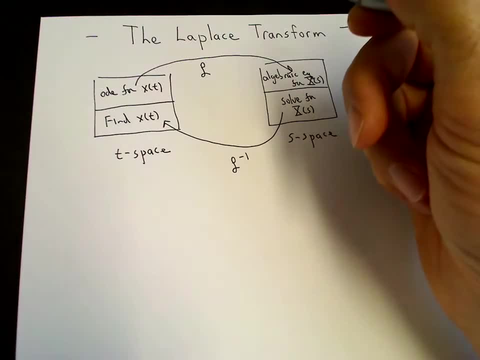 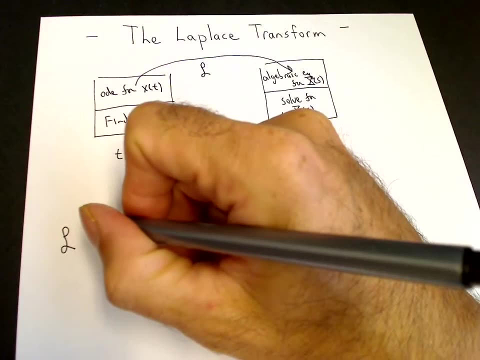 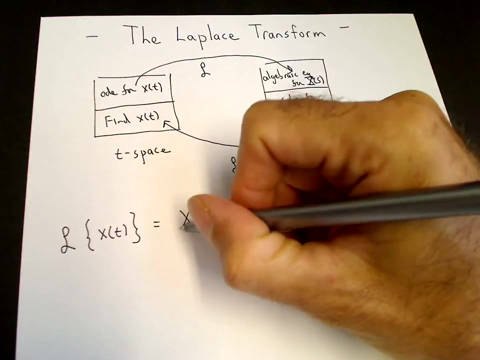 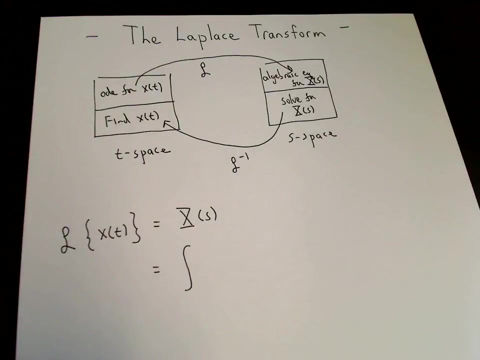 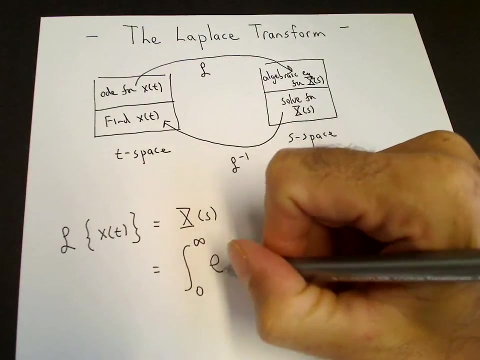 So if we have a function x of t, say, then the Laplace transform of x of t is what we're calling capital X of s, And the definition that works very well for constant coefficient equations is the improper integral from 0 to infinity, of e to the minus. 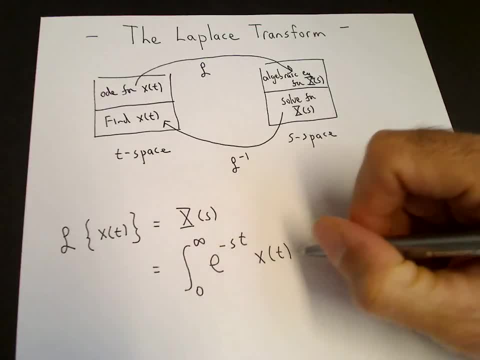 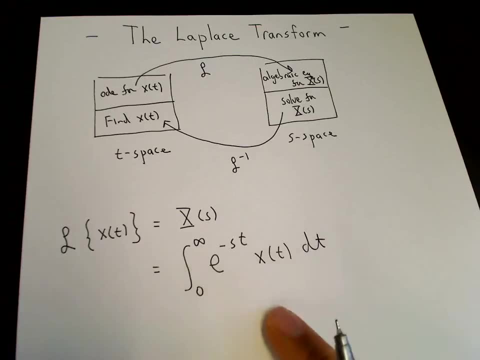 st of x, of t, dt, So we integrate over t, and the right-hand side then is a function of s. And the reason this works well is because we know that the onsatz for solving the second-order constant coefficient equation is the exponential onsatz. 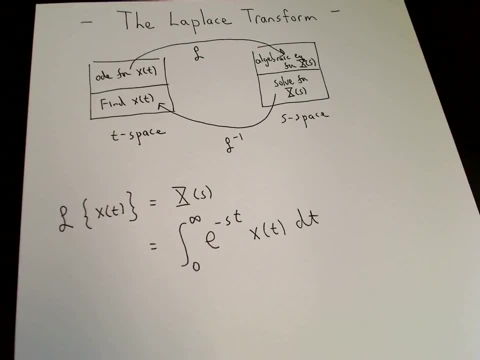 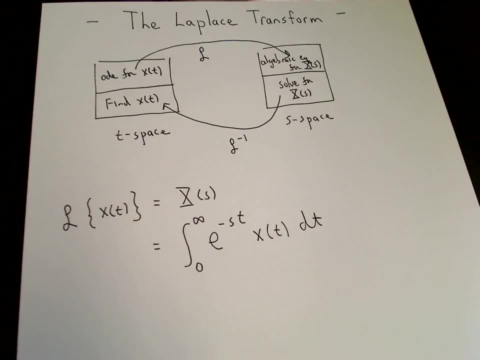 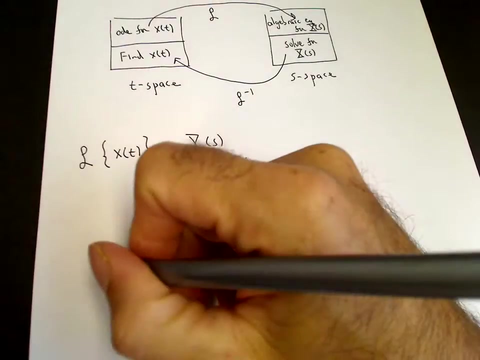 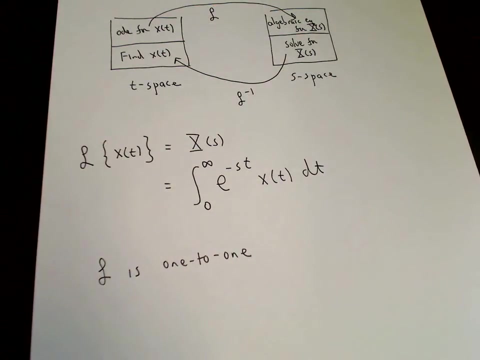 And that enables this integral to transform, And that enables this integral to transform the equation quite nicely. So we can find tables of the Laplace transform. So L is 1 to 1, which means that for every little x of t there's only one capital X of s. 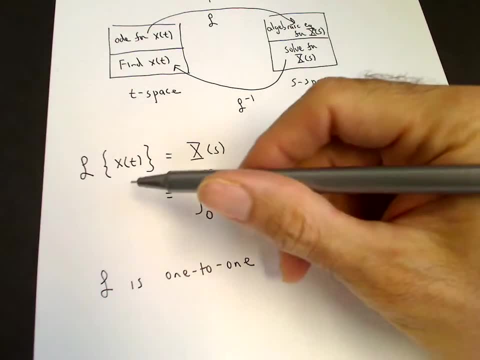 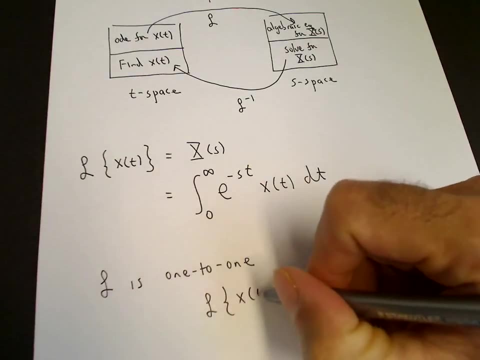 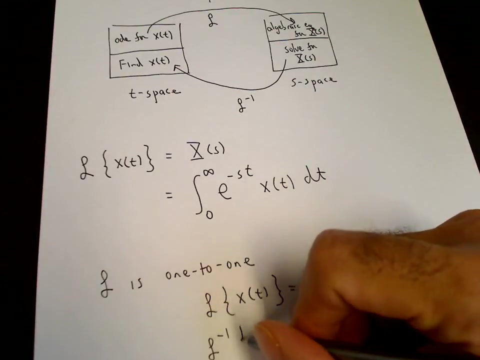 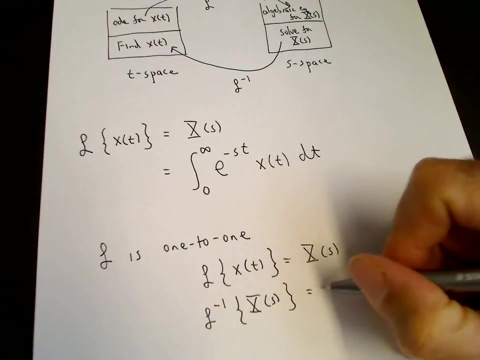 And for every capital X of t there's only one capital X of s, And for every capital X of s there's only one little x of t. So we have: L of x of t equals capital X of s And L inverse of capital X of s equals x of t. 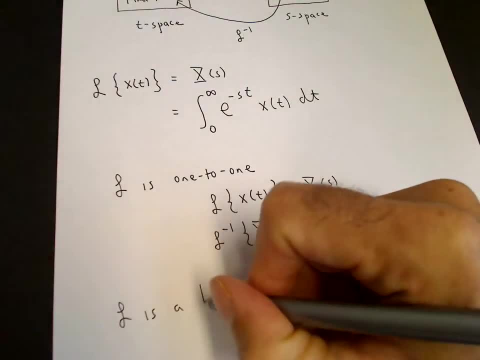 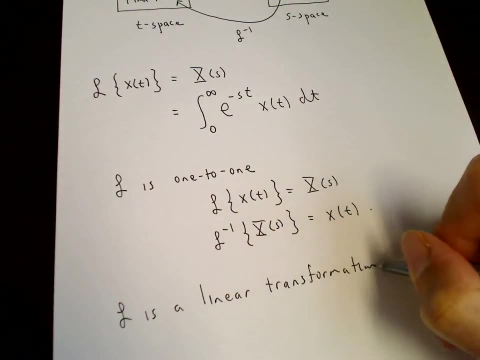 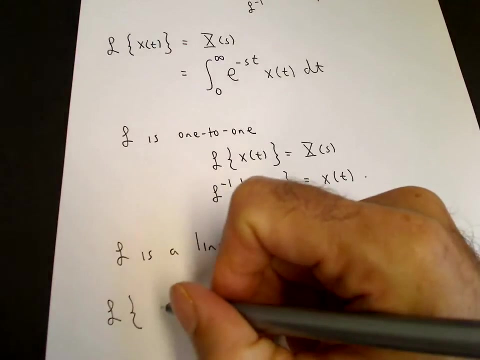 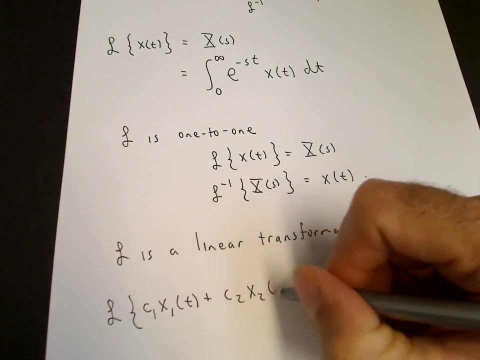 Also, L is a linear transformation And the meaning of a linear transformation is that L of c1, x1 of t plus c2, x2 of t is equal to c1. L of c2, x2 of t, x1s, x1s. 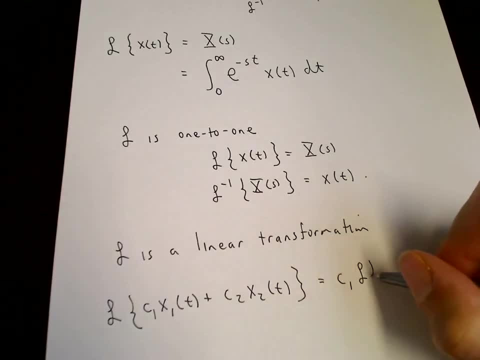 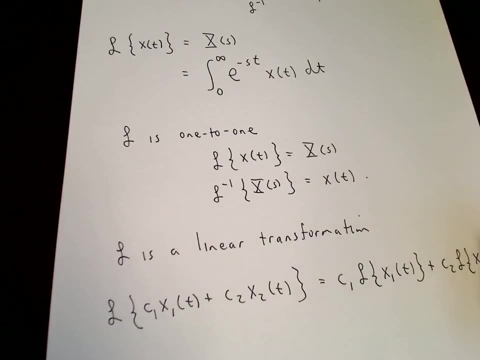 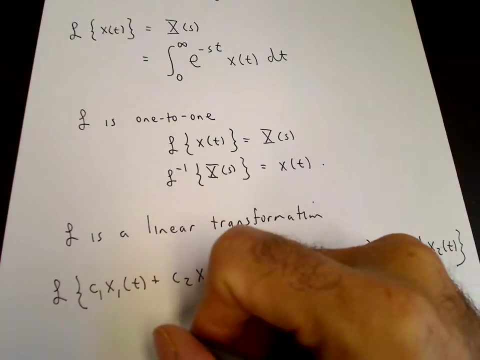 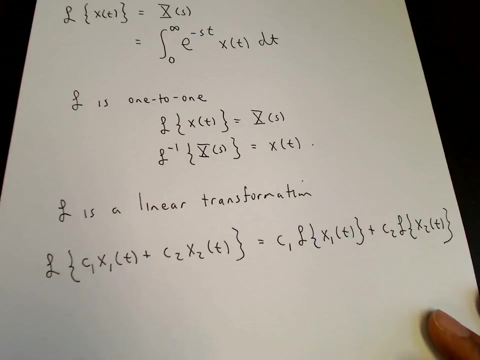 x2s, x2ls, x2ls. imbalance ofanga, point 1.. of x1 of t plus c2l of x2 of t. okay, And that's just from the property of the integral which you can prove by substitution. 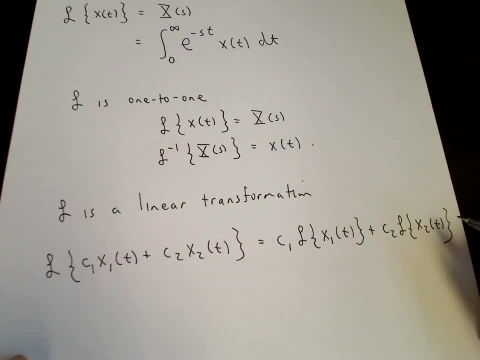 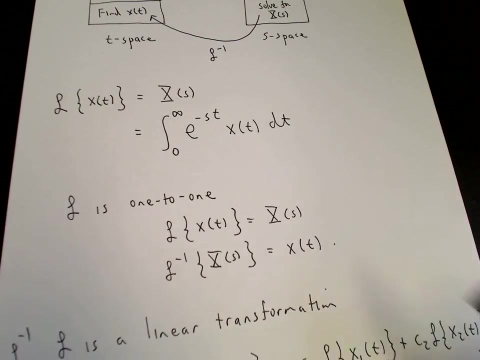 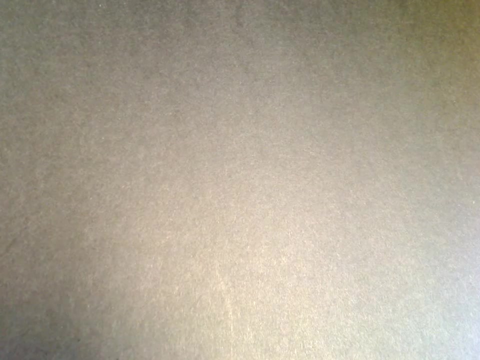 Also L inverse is a linear transformation. So L is a linear transformation and also L inverse. okay, So those are two useful properties. Okay, so L is just an integral, So we can find Laplace transforms of various functions. One does that by doing integration. 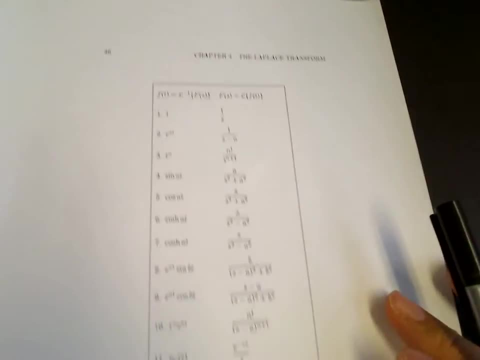 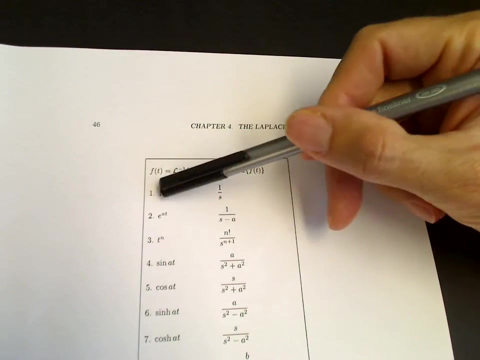 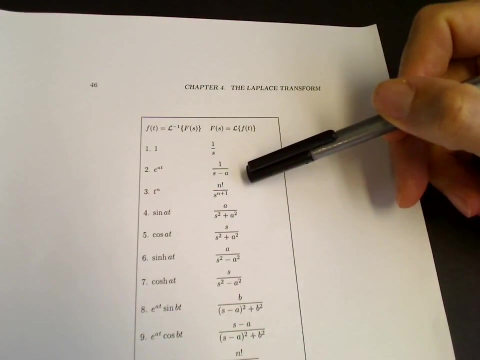 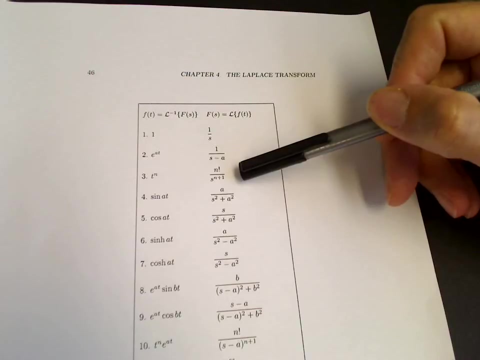 And you can end up with a table which is in my lecture now. So the Laplace transform of 1 is 1 over s, e to the at, is 1 over s minus a t to the n. where n is in positive integer, is n factorial over s to the n plus 1, and so on. 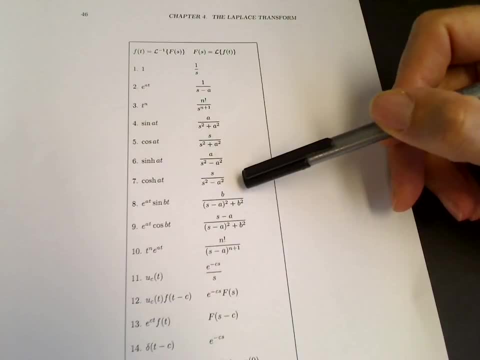 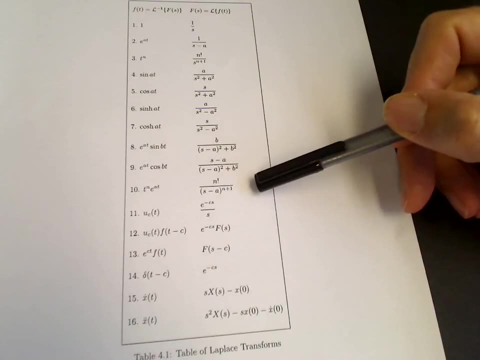 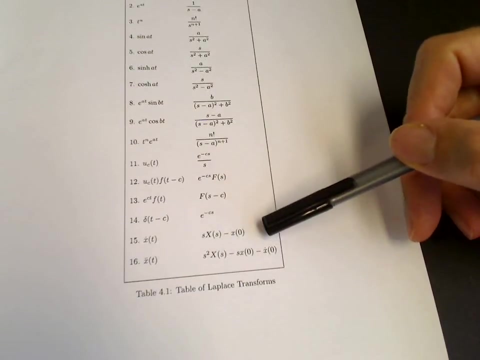 Sine cosine hyperbolic, sine hyperbolic cosine. exponential times: sine exponential times cosine Cosine. polynomial times exponential. These latter ones we'll discuss later. And then, finally, what is the Laplace transform of the derivative of x with respect to time? 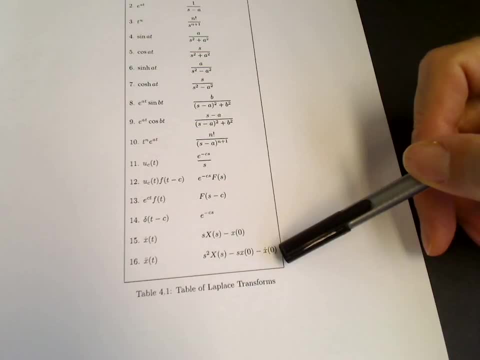 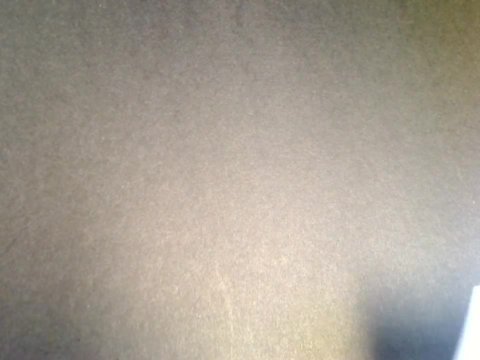 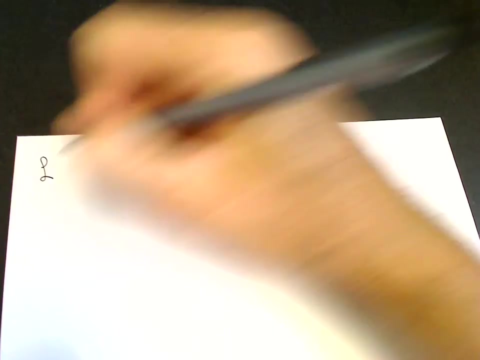 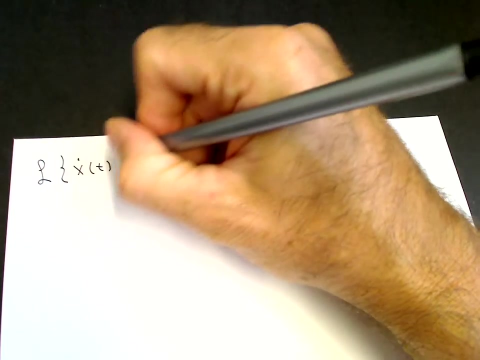 What is the Laplace transform of the second derivative of x with respect to time? Those two are needed in order to transform the differential equation. So let's let's have a look at that. If we want the Laplace transform of x dot of t, we apply the definition of the integral. 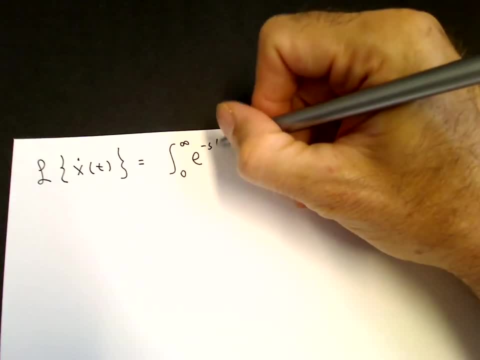 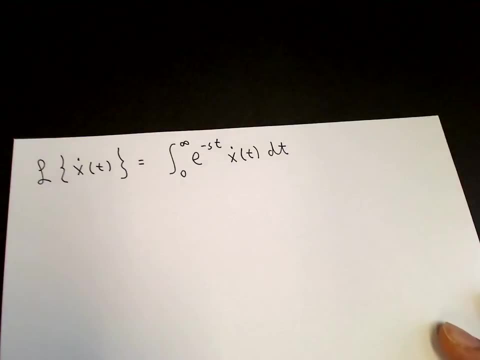 from 0 to infinity, of e to the minus st, x dot of t dt. So we want to write this Laplace transform in terms of the Laplace transform of x dot of t dt. So we want to write this Laplace transform in terms of the Laplace transform of x dot of t dt. 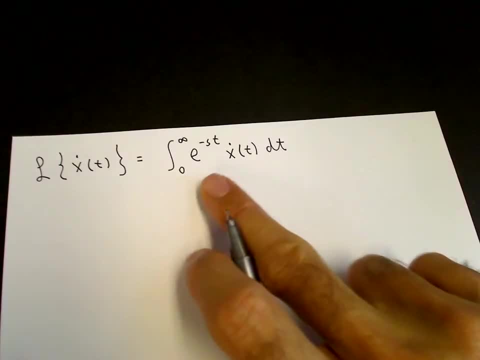 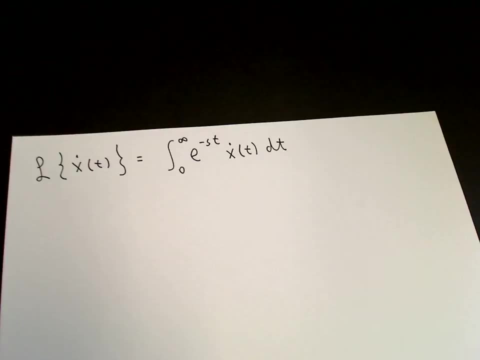 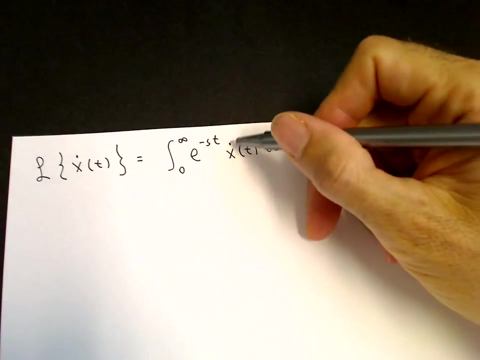 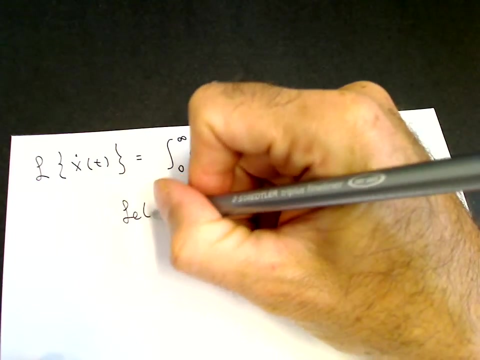 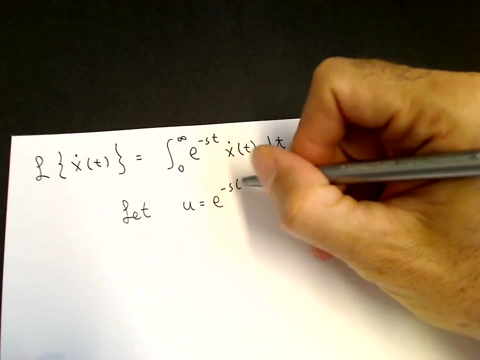 of X itself. We have exponential function times, the derivative, and immediately when you see an equation like that, you should use integration by parts, because we want to take the derivative off of X so that instead of X dot we'll have an X. so we integrate by parts. so U then we would put equal to e, to the minus st. 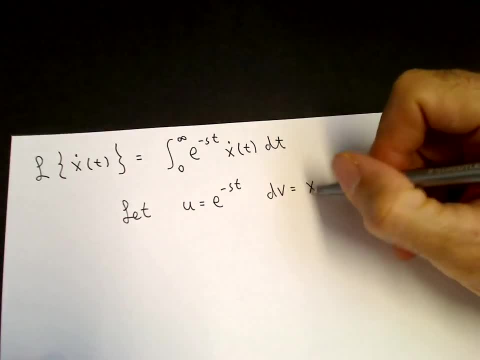 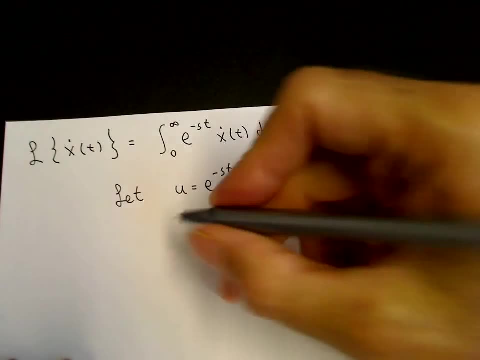 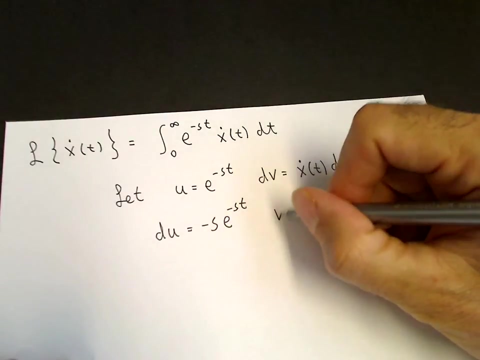 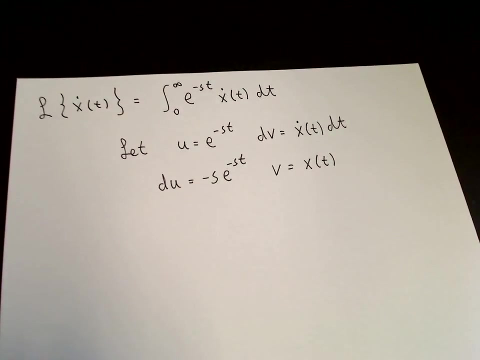 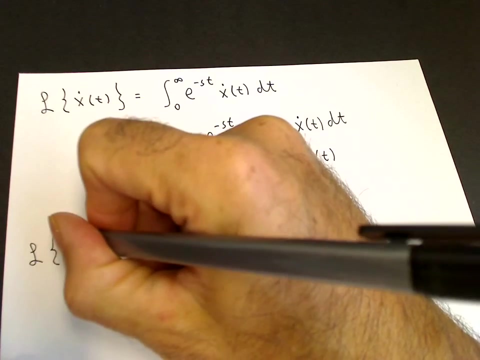 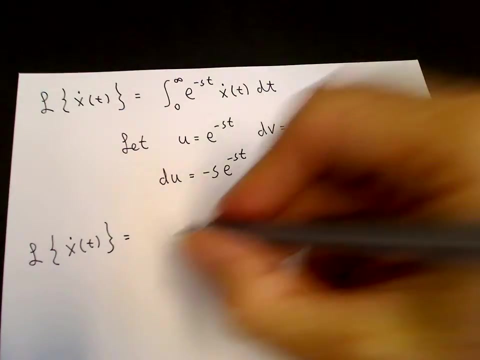 and DV would be x dot of t, dt right in a parts integration. so then Du equals minus s, e to the minus st, and V is equal to X right from the fundamental theorem of calculus. so we have then the Laplace transform of x dot becomes, with the parts integration, UV e to the minus st. 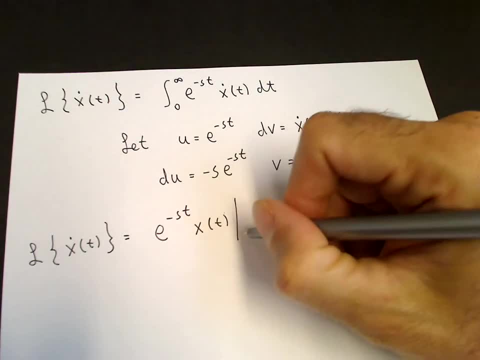 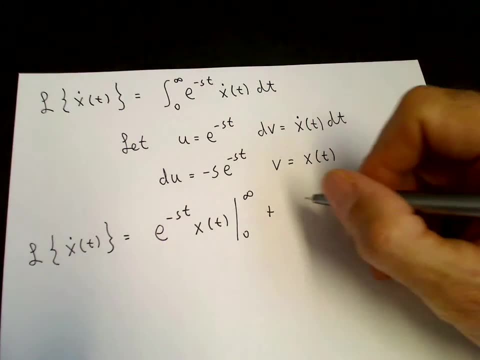 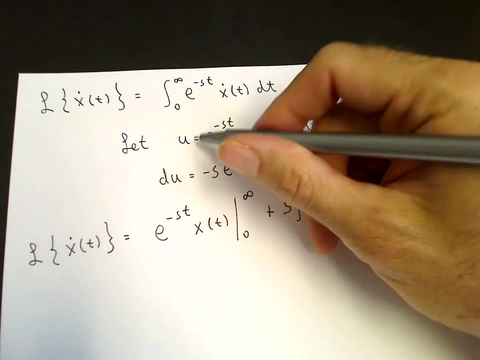 times X of T from 0 to infinity, minus the integral of Vdu. since there's a minus sign here, that becomes plus the integral from 0 to infinity s times. e to the minus st. sorry, the du, of course is u is e to the minus st. du is minus s e to. 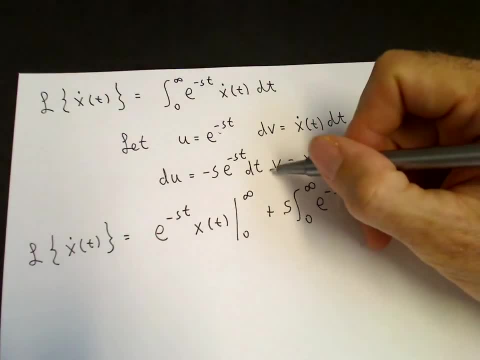 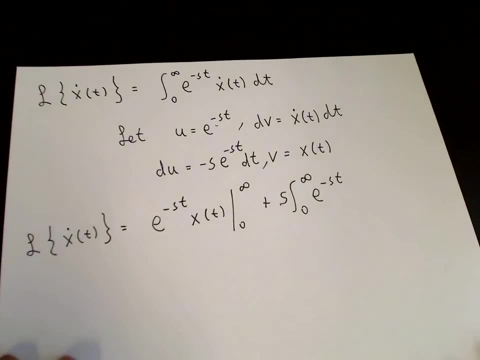 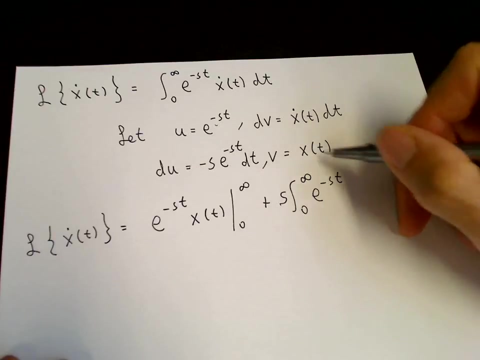 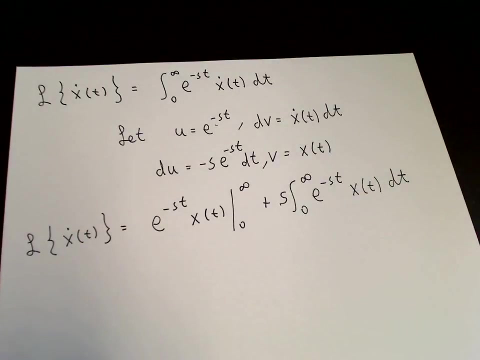 the minus st. sorry, the du, of course, is: u is e to the minus st du is minus s. e to the minus st dt. right, never forget that DT never write an integral without a DT. so I asked: from 0 to infinity: e to the minus st X of T V DT. the first term is the boundary. 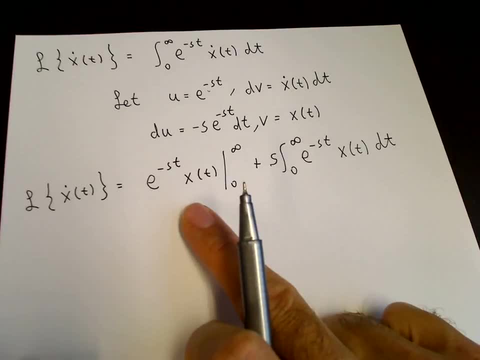 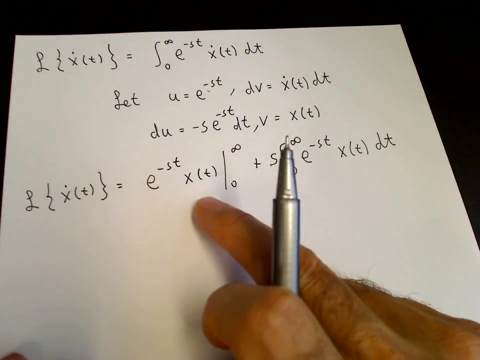 term because we're assuming that s is large enough that the Laplace transform converges. that means the integrand of the Laplace transform of X is e to the minus st times X of T and that needs to go to 0 at infinity in order for the 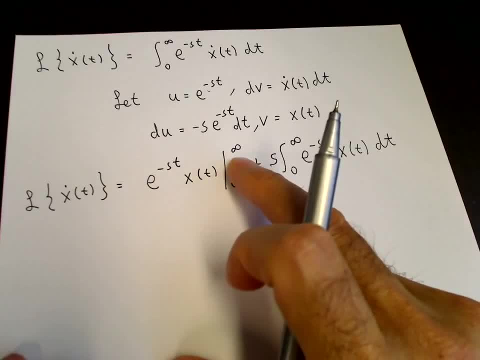 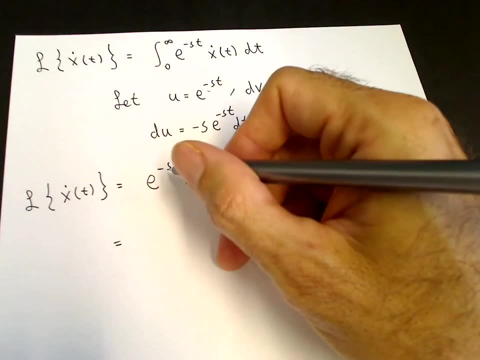 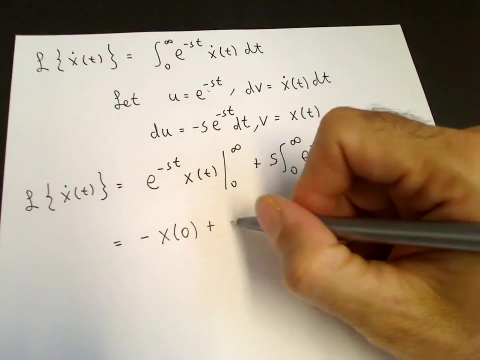 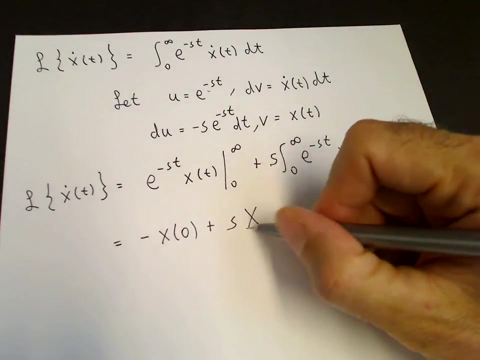 integral to converge. so the upper into the upper limit here necessarily must go to 0, and then the lower limit becomes minus e to the 0, which is 1 minus x of 0 plus s. and this is right hands. this last term here is just the Laplace transform of X. okay, so that. 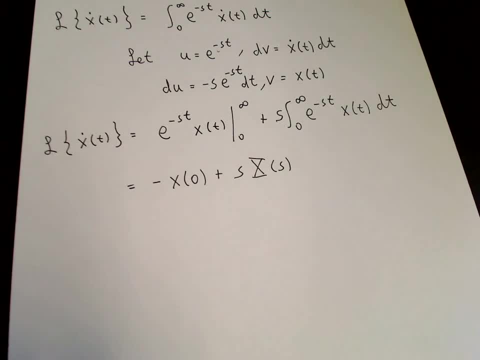 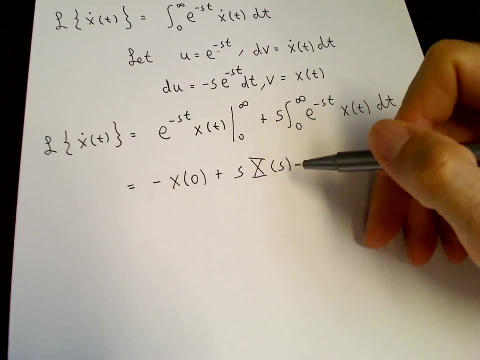 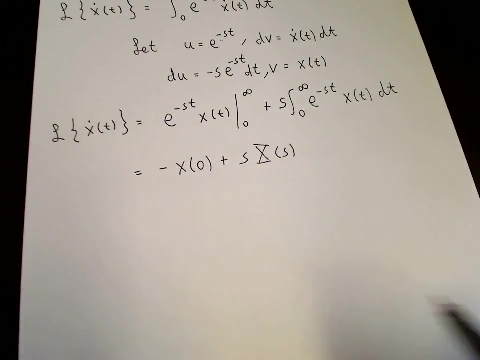 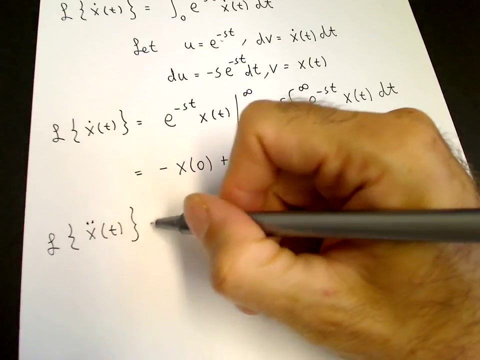 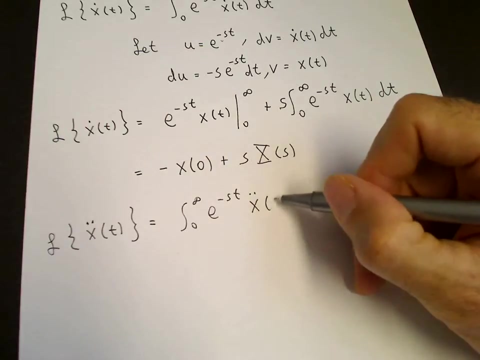 tells us how to take the Laplace transform of X. dot of T depends on the initial condition, X of 0 and plus s times the Laplace transform of x. Similarly, if we try the Laplace transform of x double dot of t, we have 0 to infinity, e to the minus st, x double dot of t, dt. 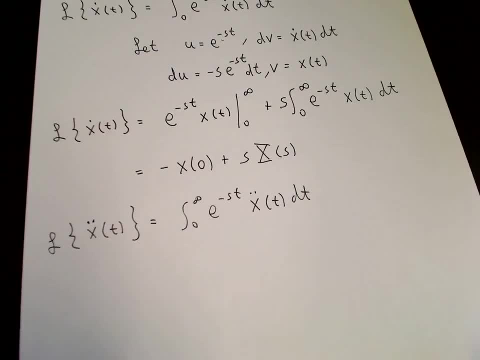 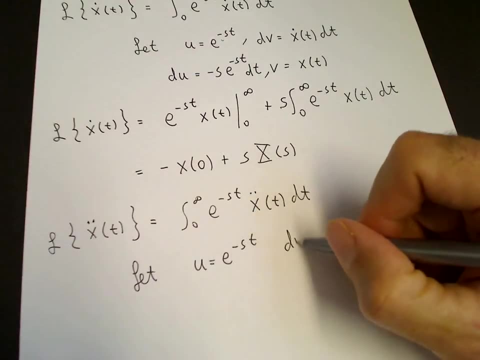 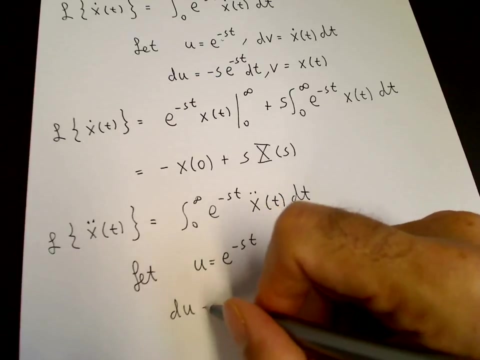 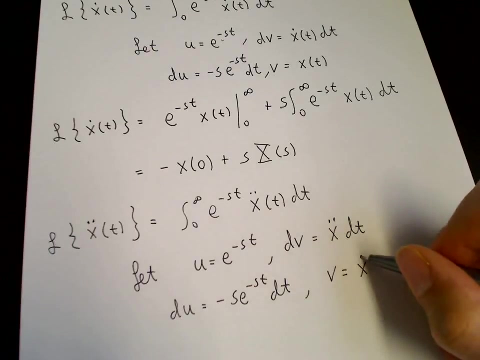 And again we can use an integration by parts. So let u equals e to the minus st dv, equals x double dot dt. So du is minus se to the minus st dt and v is x dot right. So the integration by parts.